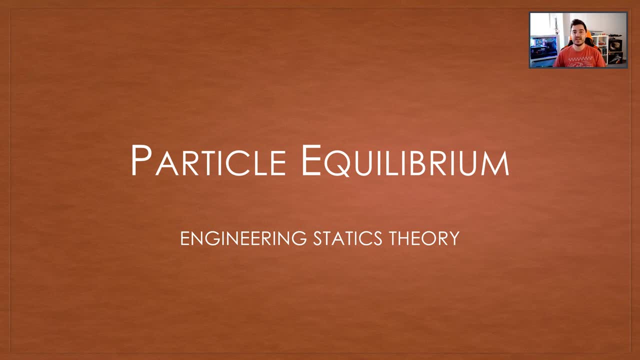 But don't worry, in this particular lecture video, we are going to discuss the simplest form of equilibrium, which is particle equilibrium. Now, for those of you at the University of Alberta, this is going to be of significant interest for you because, like I said, I like to mention what the exams have. 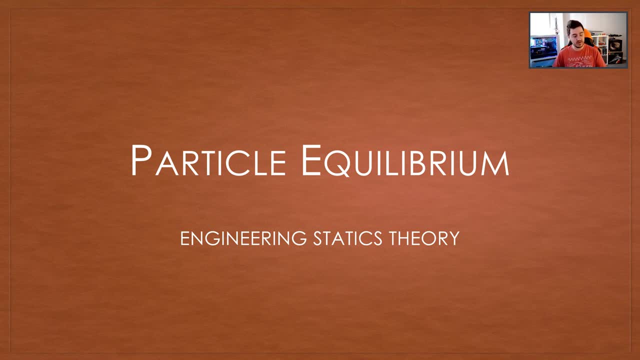 Now, traditionally midterms, the first question is always 3D vectors And we covered those last week. We're good to go. So first question: check. The second question almost always is particle equilibrium. So this is going to be your second question right here. But don't worry, secret between us, this is always the easiest question. 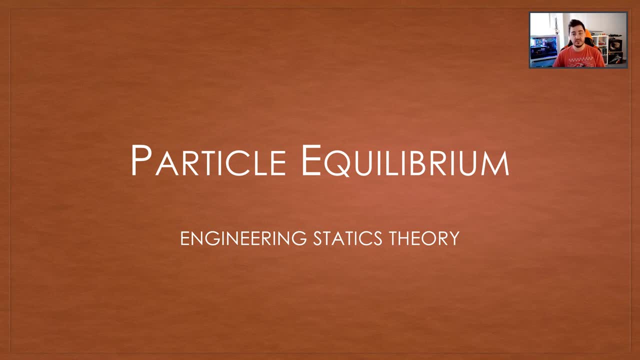 Particle equilibrium. this is going to be a short lecture because it's actually very, very simple. Now remember, at the end of the last lecture I said that we have two equations in 2D And using those two equations we can solve for two unknowns. But again, I teased you. I wasn't very nice. 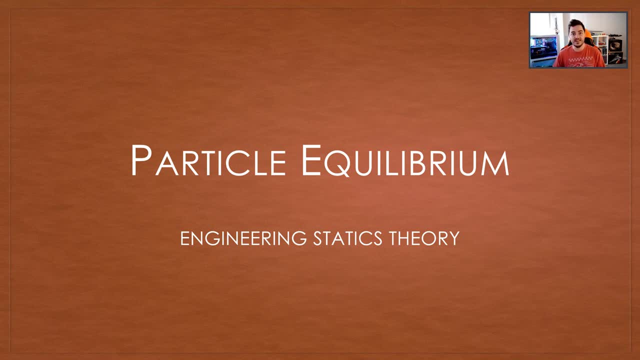 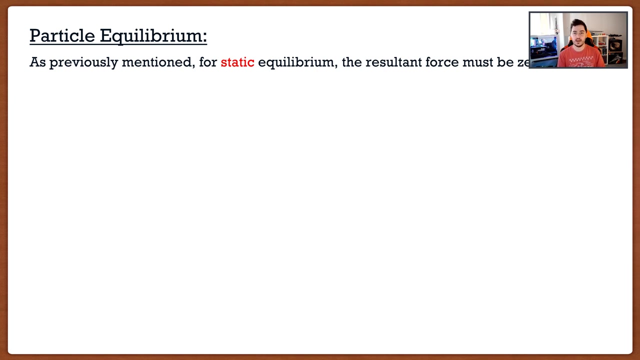 I got you guys all hyped and then left you hanging, which is kind of mean. But now we're going to talk about where these two equations come from. So that is going to be particle equilibrium. So let's begin Now. I want to emphasize here that this is going to be particle equilibrium, which means that at this point, right now, all of our forces act at the same point. 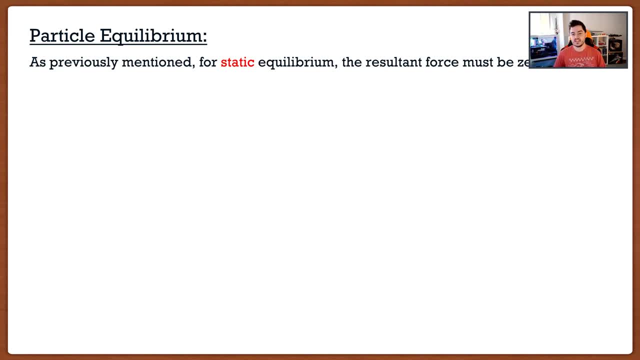 All right. so just a little disclaimer: moving forward, So for static equilibrium- remember, static we talked about last time- means that nothing's moving, It means that the acceleration is zero. And we said for this to be achievable, the resultant force must be zero. 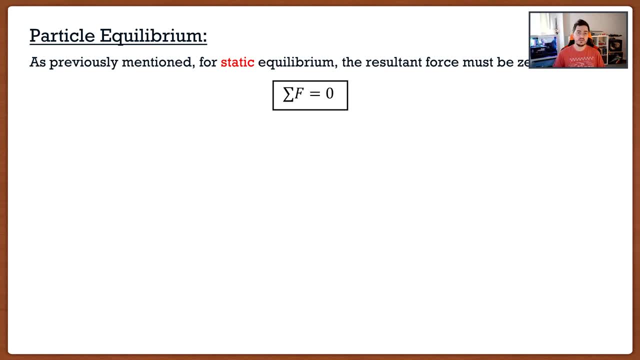 Therefore we get this nice equation where the sum of forces on a body must be equal to zero. Now we can actually expand this into two-dimensional and three-dimensional cases. All right. so for a 2D particle, if the summation of forces must be equal to zero, that must mean that all 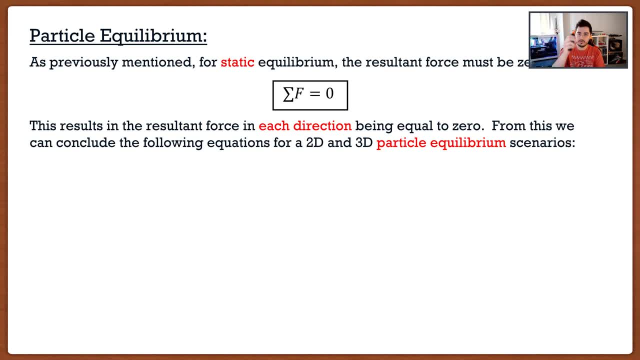 horizontal forces must be equal to zero and all vertical forces must also be equal to zero, And the same thing for 3D, except all the forces in the third direction must also be equal to zero. So this is where the equations come from. So for two dimensions, we said that both directions have to be zero. 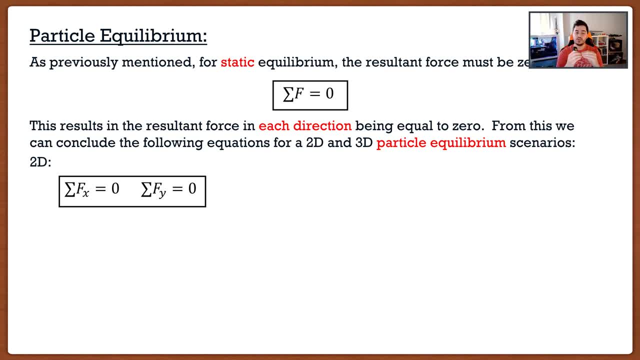 So we have two equations: The summation of the forces in the x-direction must be equal to zero and the summation of forces in the vertical direction must be equal to zero. Now for you math nerds out there. you guys know that if we have two equations, 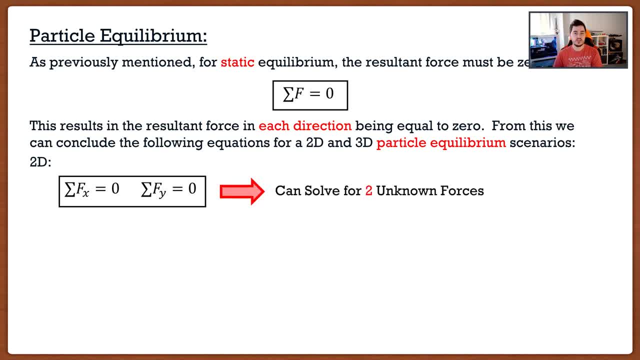 we can actually solve for two unknowns. So that's going to be kind of the first case where in 2D you guys are going to have problems where we have two unknown forces and we are going to use these two equations to solve for those two unknown forces. 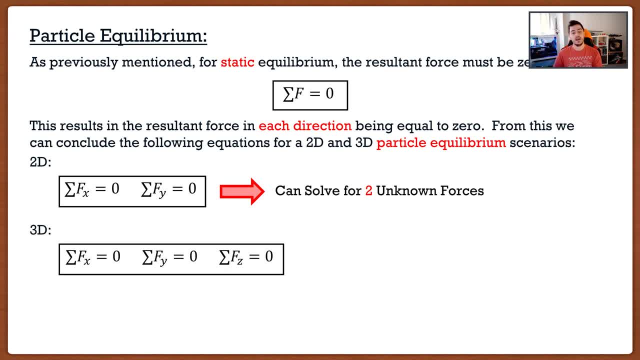 3D. like I said, it's the exact same thing, except we have that third component. So the summation of forces in the z-direction must also be equal to zero. Now, typically I do z like this or it's kind of into the page whatever you guys want. 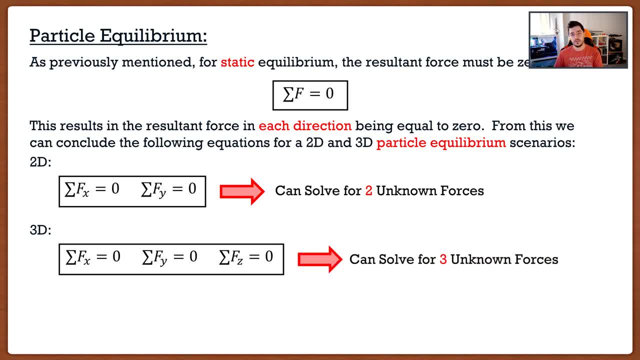 But this is nice because for 3D we can actually solve for three unknown forces Looking pretty good. Now again, I want to just clarify one thing for you guys, For those second years and even graduate students that are sneaking in here, those trolls. you guys are saying Clayton, there's actually 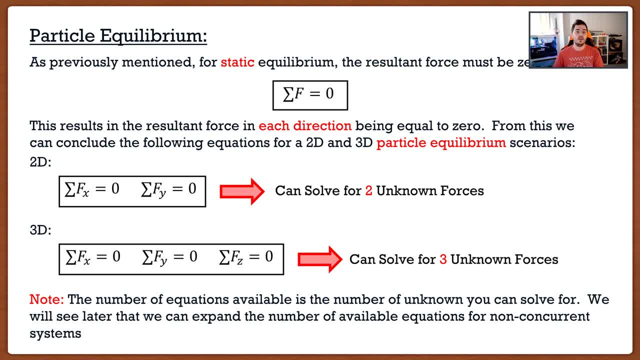 more equations. I understand, And this is why I'm very I'm emphasizing a lot that for now we're dealing with particle equilibrium. It means that all the forces act at the same point, which means that there's going to be no rotation. All right, there's the key: No rotation, No rotation. 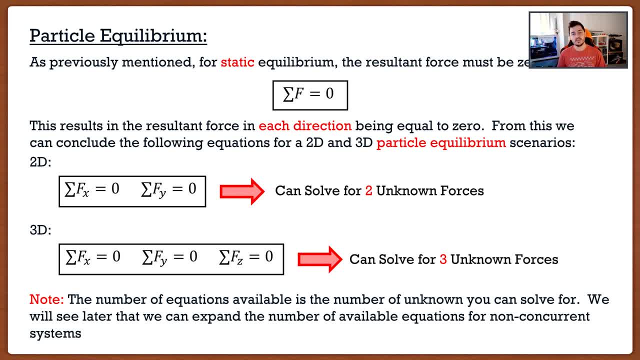 As we're going to see later on, when forces don't act at the same point, for instance, if I have a force coming down at this end and a force coming up at this end, we see rotation, And this violates equilibrium. Notice that it's not translating, it's simply rotating. 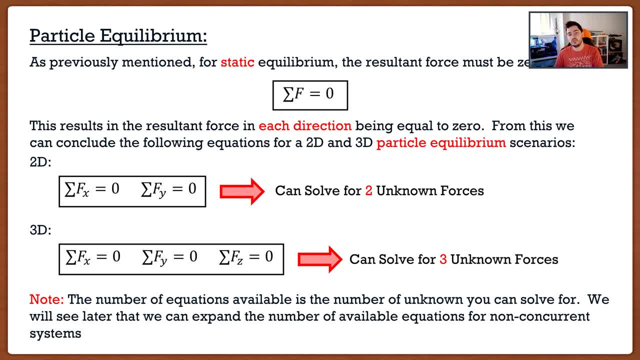 So we're going to introduce more equilibrium equations in the future to deal with that case, But for now we're not concerned with rotation because we have concurrent systems. Therefore, for 2D, two equations and for 3D we have three equations. 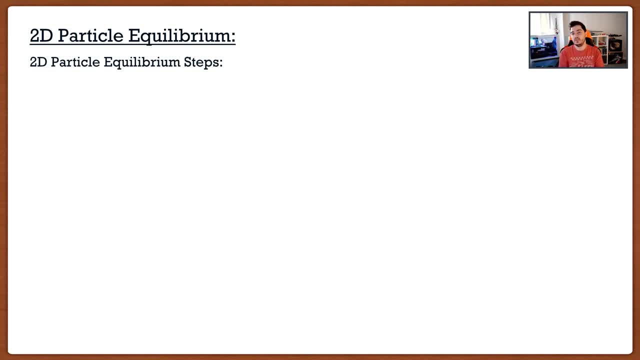 So let's discuss 2D. If you guys understand 2D, then 3D is going to be the exact same. So this will give you a brief understanding of what exactly we're going to do. Now, when we're dealing with particle equilibrium, the formula, the process can actually be broken. 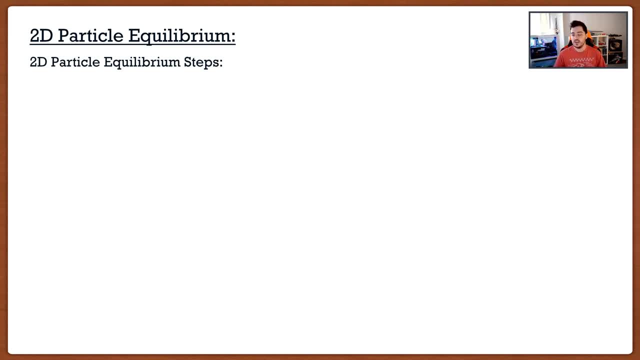 down into a series of steps and these steps never really change. There might be a little bit extra in each one of the steps if you have, let's say, a pulley or a spring, like those special members we talked about, But for the majority it's going to be nice, easy and very basic. I know that. 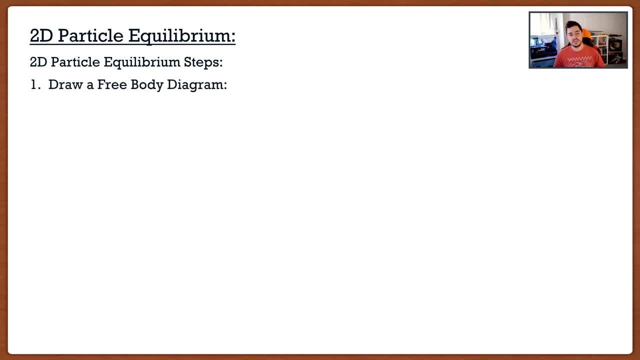 everybody likes that Easy and basic right. So the first step always going to be draw a free body diagram. I hinted at this last video. You always want to draw a free body diagram because if you don't, you're going to get marks taken away. Usually they're worth about 20% of the 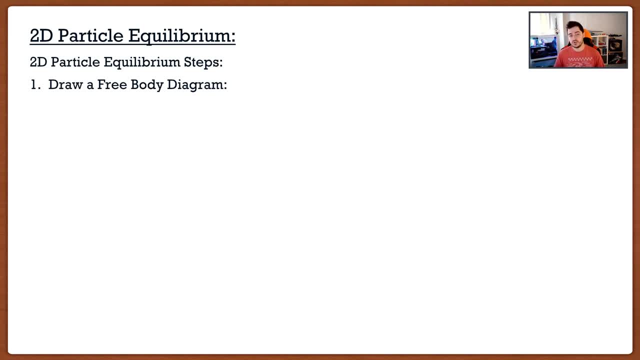 question. So sometimes it can be quite sizable. So you're going to want to draw that free body diagram. But we showed you free body diagrams. You guys said: you know what, Clayton, this is pretty easy and that's great. It means that you guys are going to get those partial marks, really simply. 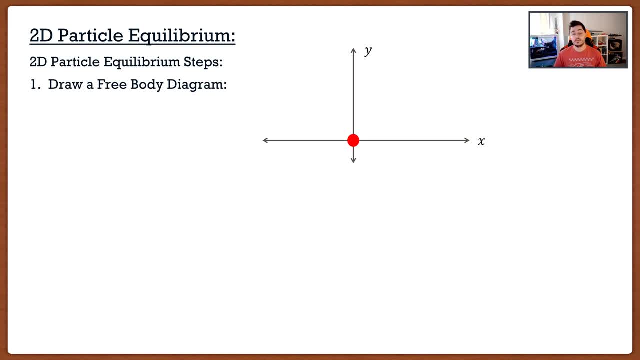 So let's say that we have a 2D case and at this point we have three forces acting on it. So again, the first step: in free body diagram, draw all the forces. So in this particular case I have 100 units of force going right, I have to. 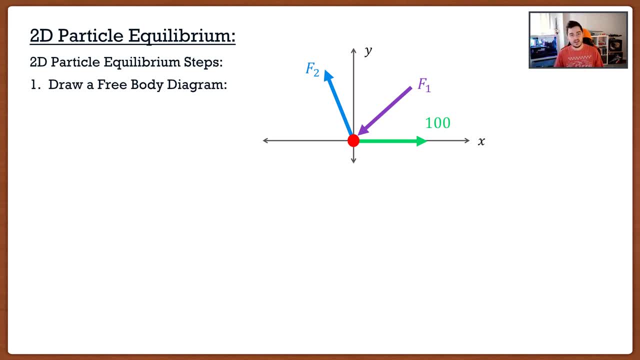 check sometimes. I did that in my driving exam. The instructor was scared shitless where they said turn left And I had to on the steering wheel. I had to do this to make sure I knew which way left was. But we have 100 units of force. I want to say newtons, but that will just scare the 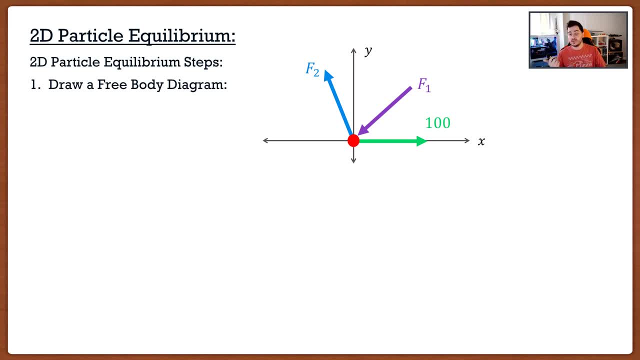 American viewer. So I'm just going to say 100 units of force going towards the right and we have two unknown forces, F1 and F2.. So again, first step in free body diagrams: draw out the forces. The second step is draw out any dimensions. Now, the beauty of particle equilibrium is everything. 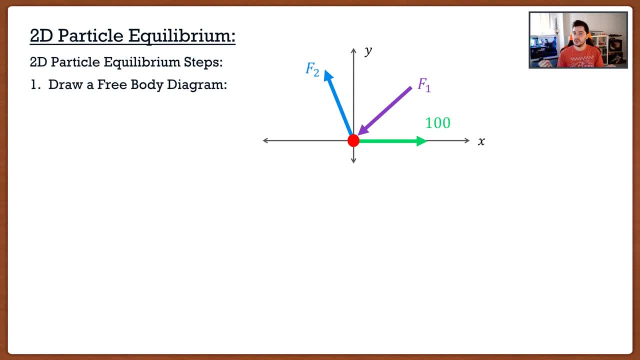 acts at the same point, So you'll never have any length dimensions at all. So for here we'll have angle dimensions. So we're going to say that F1- we know- acts at 40 degrees and F2 acts at 40 degrees. So after that, the next big step is going to be finding out the force components. 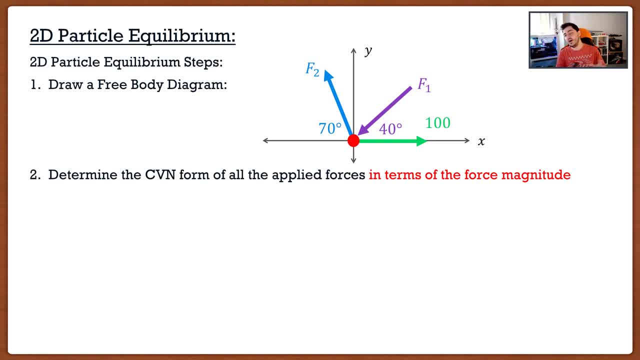 of all the forces. So this is where week one and week two kind of come into play. here is we have to take our forces and convert them into Cartesian vector notation. So we're going to say that F1, looking at it, we can split it up into its x and y components, where the x component 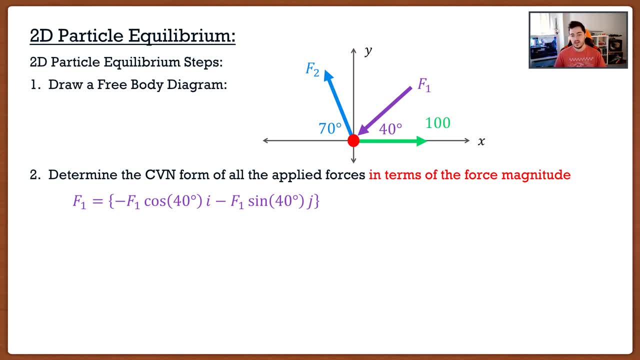 is going to be negative one times F1, because again it's going in the left direction. so it is going to be negative multiplied by cosine of 40 degrees. And then the y component is going downwards, so it's going to be negative and it's going to be F1 times sine of 40 degrees. 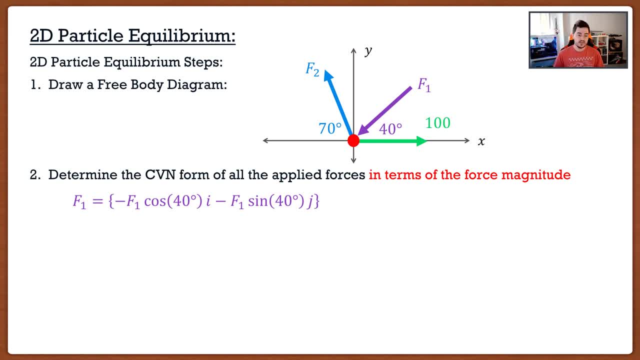 So if we look here, we know that F1 is actually an unknown, So we have the components ready, but there's still an unknown inside of those components. For F2, it's going to be the same thing. So F2, it's going to the left. therefore it's going to be negative in the x direction. So we're going to say negative F2 times cosine of 70 degrees. that's negative. 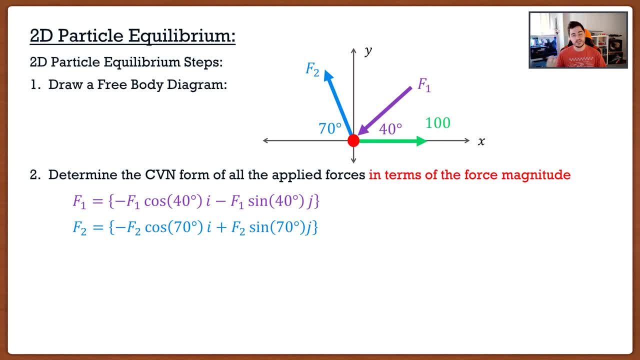 And since it's going upwards it's going to be positive. So we're going to say plus F2 times sine of 70 degrees. So now I have all of my unknown forces in Cartesian vector notation. Now the hundred is very simple, we know it's simply just going horizontally. but if that hundred was, 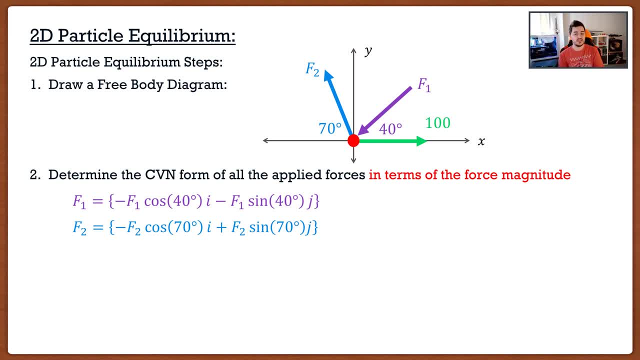 angled in any sort of way. we'd also want to include that force into Cartesian vector notation. Now you guys are saying, Clayton, this is pretty trivial, I don't know why I have to express them, them in Cartesian vector notation. and I'm going to let you guys in on a secret. You don't If you. 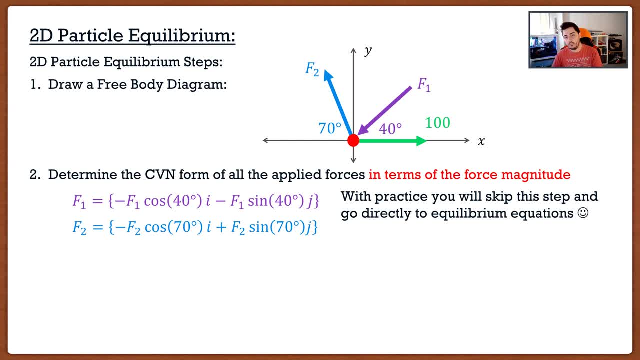 guys are very comfortable at finding force components, so fx, fy, etc. you guys can skip this step. The reason why I'm showing you guys this step, even though it's really tedious, is it'll make much more sense for the three-dimensional case. Usually, professors skip this step when 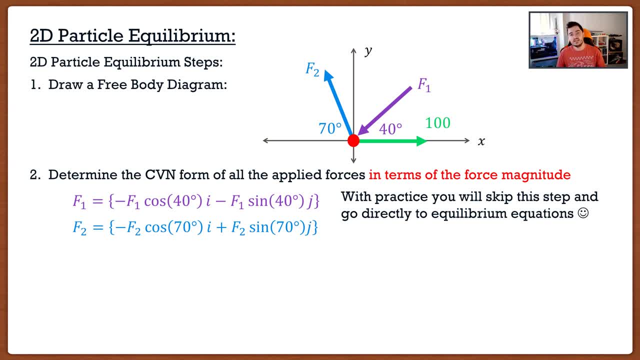 they teach it to you guys and students saying all right, 2d, nice and easy. Then you guys get to the exam and it's 3d and no one knows what to do. So this is why I'm showing you guys this step. 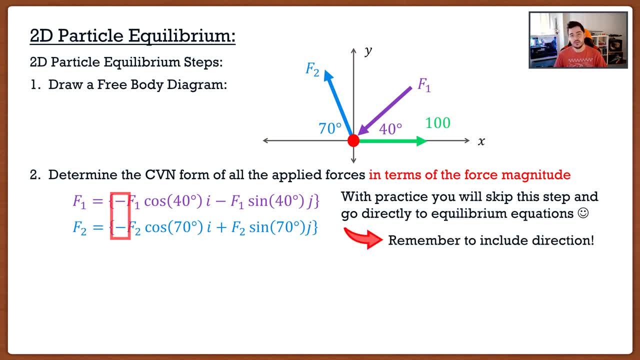 So the final thing I want to mention is make sure you guys include direction Again we talked about for both f1 and f2. they're both going to the left. therefore we know that it's going to have a negative sign on those x components. So once we have all those, we can use our equations of 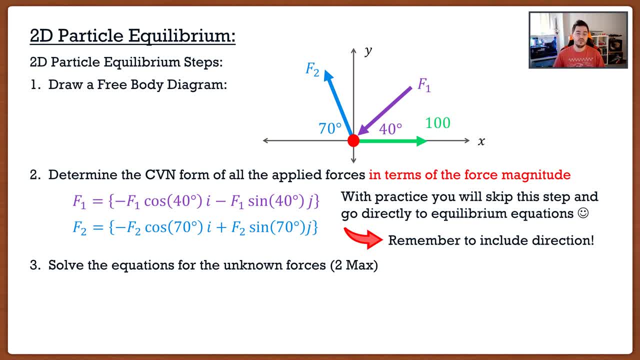 equilibrium to solve for the unknown forces. So remember, in two dimensions we have two equations: summation of forces in the x direction must be equal to zero and the summation of forces in the y direction must be equal to zero. So we're going to start off with the x direction. 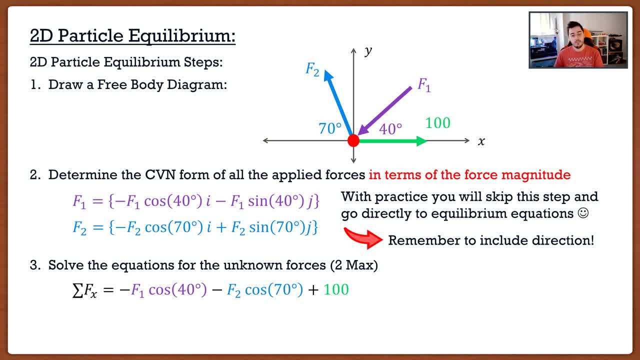 And I get negative f1 times cosine of 40 minus f2 times cosine of 70 plus 100.. And you guys may be saying, whoa, hold on there, big guy, where did you get those numbers from? Well, if we're dealing with the x direction, we're dealing with the x component of all the forces. So what I did is I: 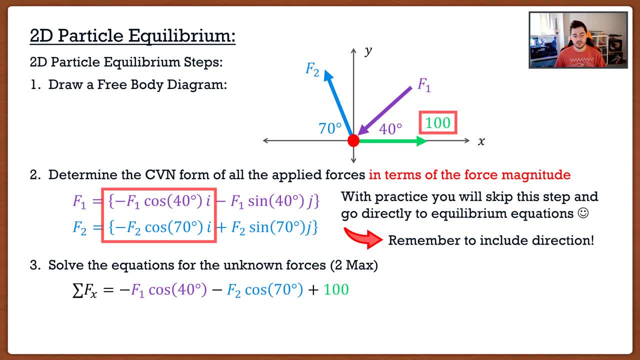 looked at the two x components or the i components of f1 and f2.. I threw them into the equation and then I have to also remember that I have the third force, 100, which is going to the right. So I also throw that into the equation as well. So it's again just all of the i components added together. 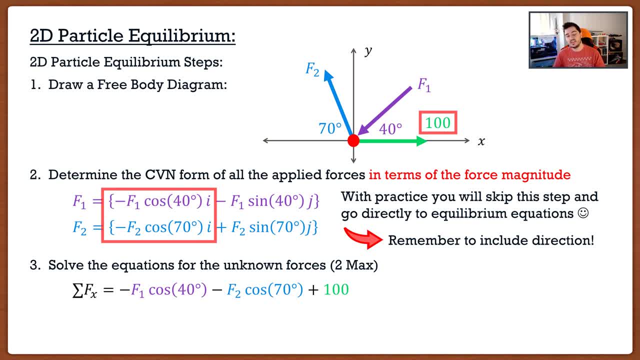 Now, in order to be in static equilibrium, remember that summation of forces has to be equal to zero. So we know that this chunk here must be equal to zero. So now we have one equation. How do we get the second one? Well, we take the summation of forces in the y direction, and it's much easier. 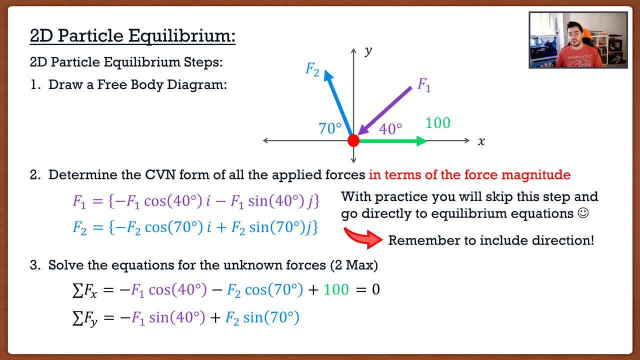 because we only have the two components. Again, you guys may be slow down, chief, Where did you guys get those components from? Well, I got them from the j components. So all I did was I took those two j components, added them together If the 100 had a j component. 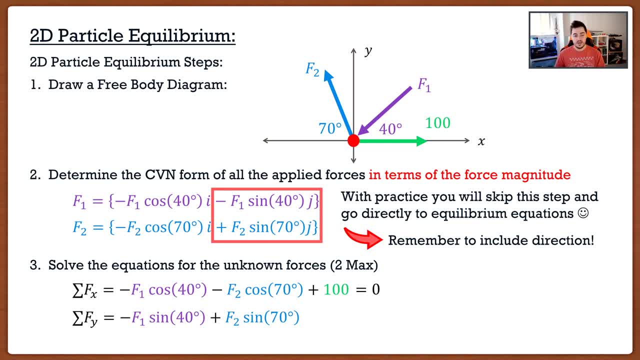 I would include that too, but, as we can see, it's perfectly horizontal. And again, to maintain static equilibrium, we know that this must be equal to zero. Now again, this is where the math nerds shine, because we have two equations, two unknowns. we can solve for f1 and f2, and I get f1 to be 100. 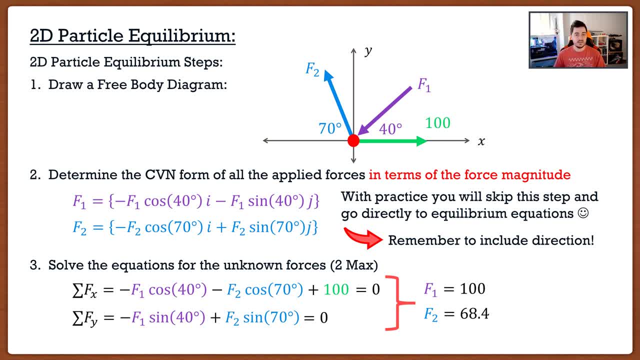 and f2 to be 68.4.. That's it. That's all you guys do in particle equilibrium. That's why students are doing this. It's fairly simple. Now you guys may be saying: all right, Clayton, this is great, I look. 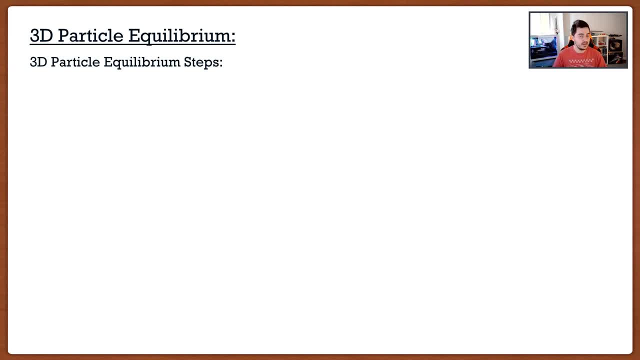 forward to this question And then the prop hits you with a 3d question. You guys are thinking, ah shit, Now what do I do? Well, 3d is going to be the exact same steps. There's only one thing that makes it harder, and that is determining the vector components. That's it. First step: draw a free body. 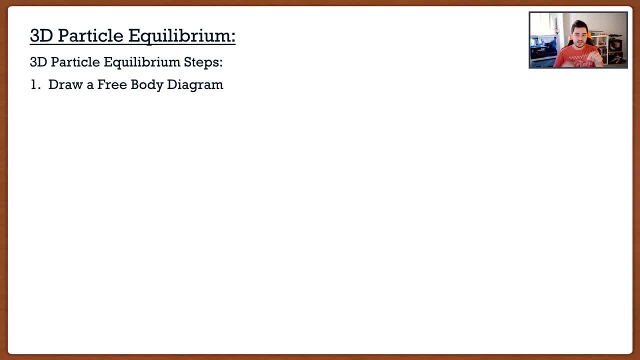 diagram Again for particle equilibrium. you're basically just drawing a dot and you're drawing all the forces on it. It doesn't have to be to scale or anything like that, but just make it as neat as possible. So again, free body diagram, easy marks: That's the bread, and 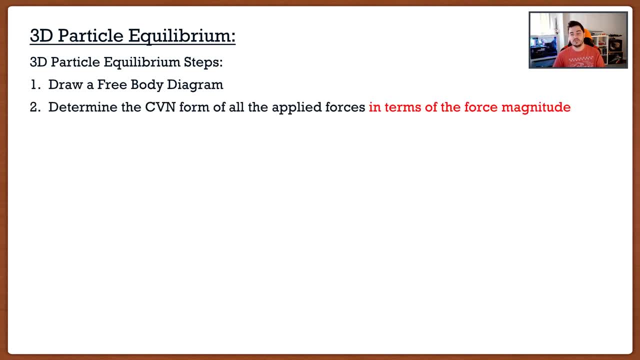 butter of part marks right there. Free body diagram. The second part is where things get a little bit more difficult because we need to take all of our forces and throw them into cartesian vector notation. Remember 3d can be quite difficult because we have three different cases that we have. 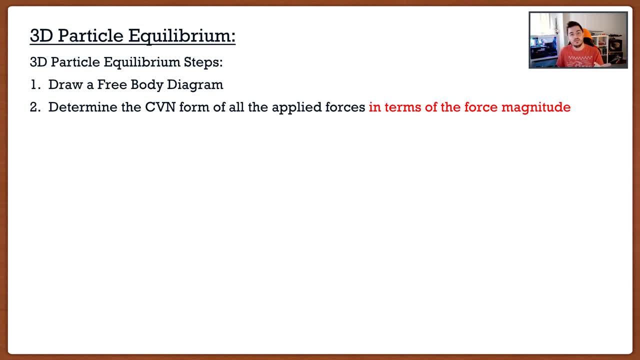 to consider The trigonometry case, the coordinate direction angles, as well as the position vector case. Now, for me, I always find the easiest is to determine the unit vector of those three components. The reason why? Well, we know that a force vector can actually be expressed as the 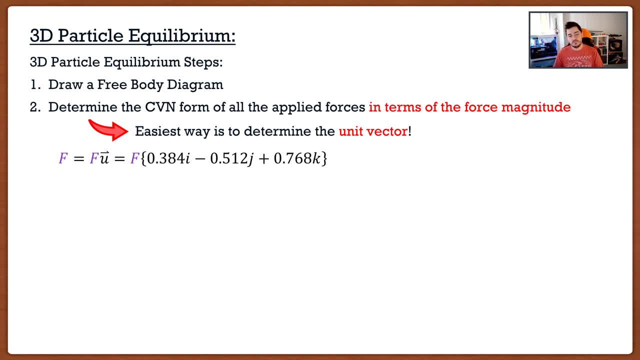 force multiplied by the unit vector. Therefore, in this particular case, I have my force f multiplied by a vector, So this vector right here, this is actually going to be the unit vector. If you guys know the unit vector, you guys are good to go, because we can actually expand this out into 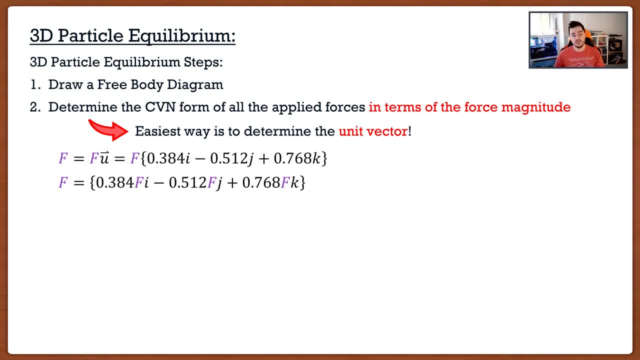 the following. So therefore, we know that our x component would be 0.384f, Our y component would be negative 0.384f, Our y component would be negative 0.384f, Our y component would be negative 0.512f, And then our z component would be 0.768 times f. Once you guys have the forces into 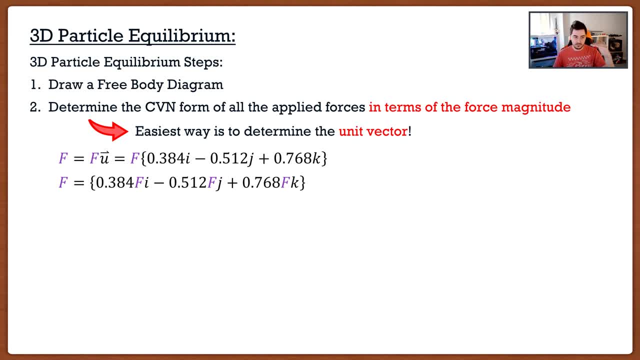 cartesian vector notation. then the rest is simple. When you go to your three equilibrium equations, you just pick out the components and place them accordingly, And this is why in the previous slide I showed you guys the vector into cartesian vector form For 2d. it's very simple to go right to the 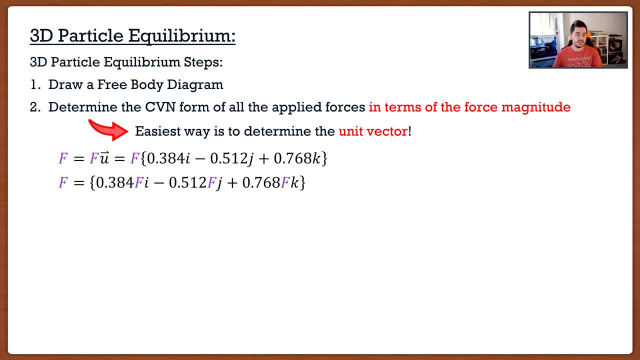 equilibrium equations, because you can very easily tell the components in each direction. But again, this screws you in the 3d case, because in 3d it's not so obvious where the components come from. In 3d it's much better to write them into cartesian vector form, because then when you guys get to the 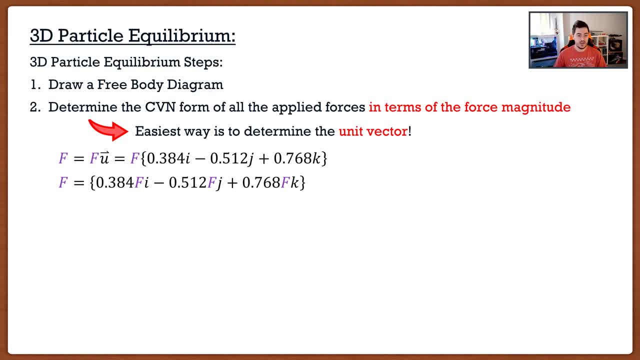 next step, which is the equations. you guys can just pick and choose and go all the way. So again, these three components, these are going to be the components I use in my three equilibrium equations. So I have, if I have, all my forces in cartesian vector notation, well then, I can go down and I can. 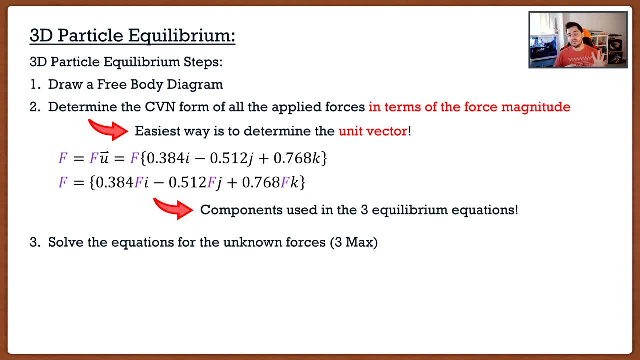 solve for my three unknown forces. So remember, in 3d we have three equations: summation of force in the x, summation of the forces in the y and summation of forces in the z, and they must all equal zero. So we have three equations, which means we can solve for. 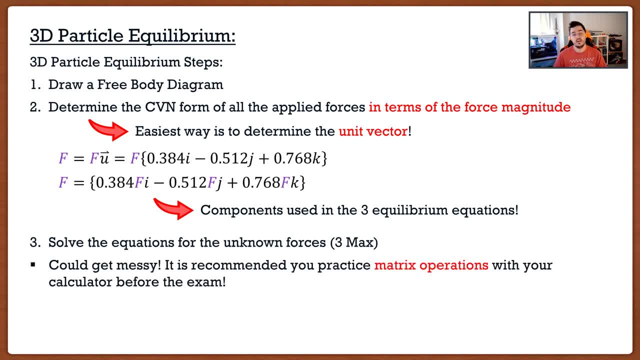 three unknowns. Now this is where you guys should get good with your calculator and it's like that: get good like g-i-t-g-u-d. get good with that calculator, because what's going to happen is it can get kind of messy: Three equations with three unknowns. if you guys are doing it by hand, it's. 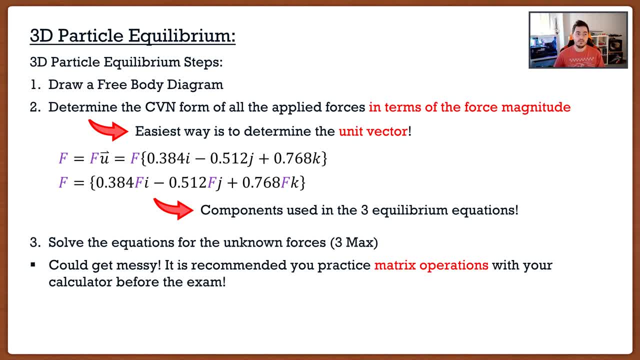 going to be a lot of work, But again you guys can all do it. you're very, very smart people. but again, the name of the game in midterms and exams is speed running. You guys want to speed run through that exam so that you have time to finish A lot of the times, and this is the biggest dick move. but 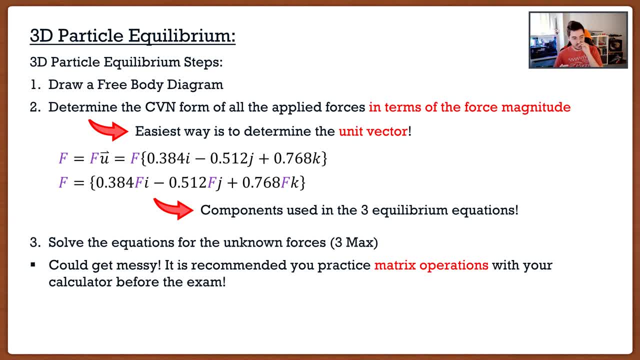 I've seen it so often. the fourth question. the midterms at the University of Alberta are four questions. The fourth question is almost always the easiest. almost always The problem is students spend so much time on questions one, two and a part of three. They always lose so many marks it's. it's pretty cringeworthy, if I'm being honest. So anything you. 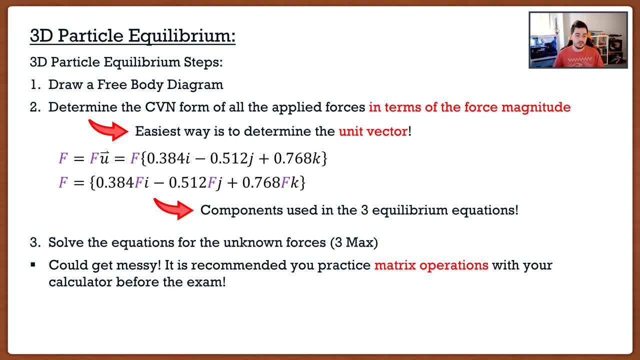 guys can do to make the exam quicker. that's what you're going to want to do. So what I recommend is, if you guys have this system of equations- three equations, three unknowns- solve it in your calculator, put down the answer and then move on. The best case scenario is, let's say, you move on. 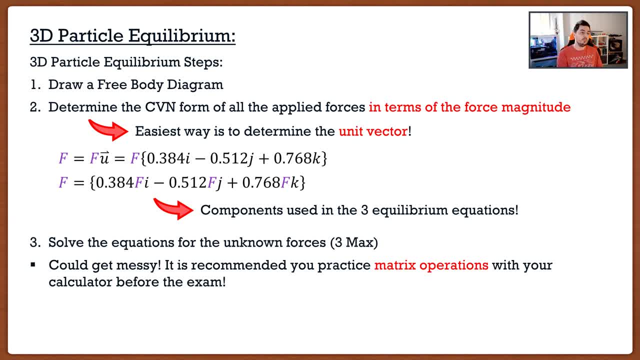 you finish the exam and you have some time left, Well then you guys can go back to this question and then try and solve it by hand, Maybe get some more part marks, something like that. but if you guys can solve in your calculator and get a, 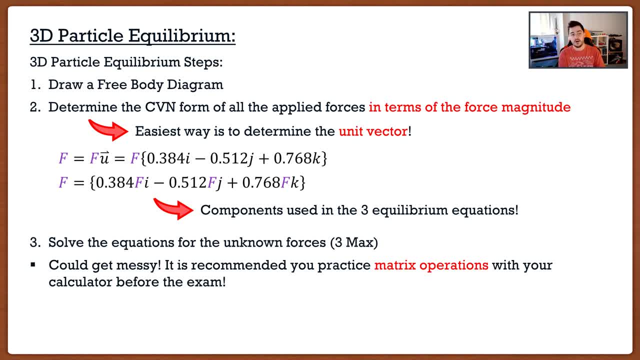 correct answer. that's going to get you guys a lot of marks right off the bat, and then that extra proof- well, that won't be worth as many marks. So maybe skip it for now and come back if there's time. Remember you want to try and attempt every question Again usually. the fourth question is the. 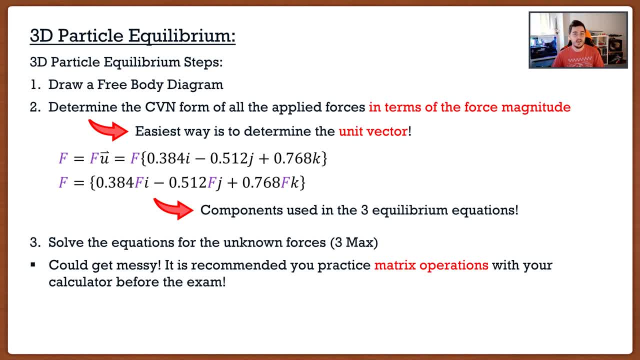 easiest and students don't have time to even get there and then they get upset because they think, oh, I missed out on easy marks. The name of the game is part marks, so you want to try and do that. Do what's going to help you and then you get the answer. Maybe you don't have time to do as much as possible. 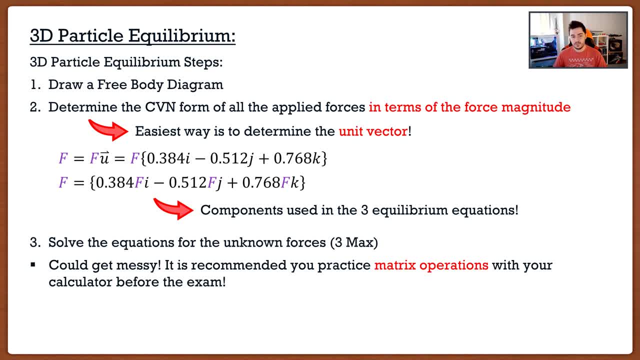 But yeah, that's 3D and 2D particle equilibrium. The worst thing they can do is throw you the special cases, So maybe a pulley or maybe a spring, something like that. but don't worry, I'm going to show you guys examples. 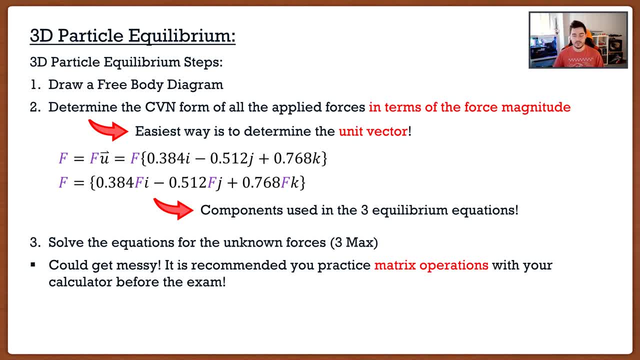 So, as always, the best way to learn, in my opinion for this course, is through examples. So this is going to be kind of a beefier video, or I'm going to have three examples down below. I'm going to have two for 2D and one for 3D. 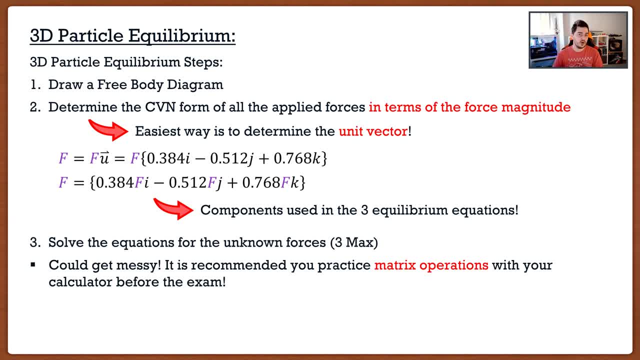 3D is very simple. usually in 3D, if they give you a 3D scenario, They're not going to to give you guys a special member like a spring or a pulley, so that one's going to be pretty straightforward, just more time consuming because it's 3d. but i'm going to have two examples in 2d: 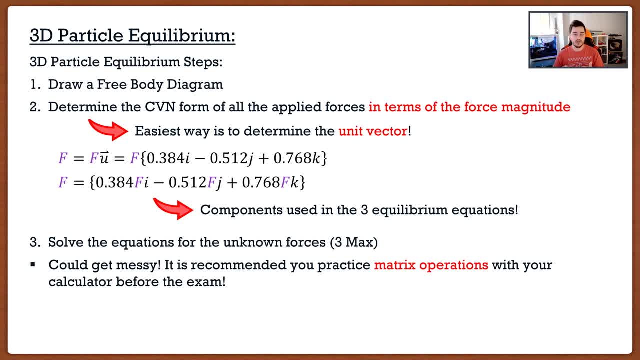 one's going to contain a pulley, so you guys know exactly what's going on there, and the second one's going to contain a spring again. springs students seem to hate the most, but it's actually one of the easier cases because we have a nice sexy formula to basically give us one of the forces. 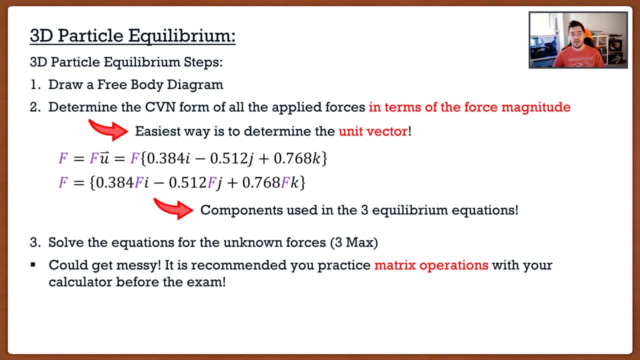 right off the bat. so, yeah, that's it for this video, guys. i just want to thank you guys all so much for listening and i just want to tell you guys, don't be stressed, be happy. engineering's supposed to be fun. so if you guys are finding yourself maybe a little bit stressed, just take 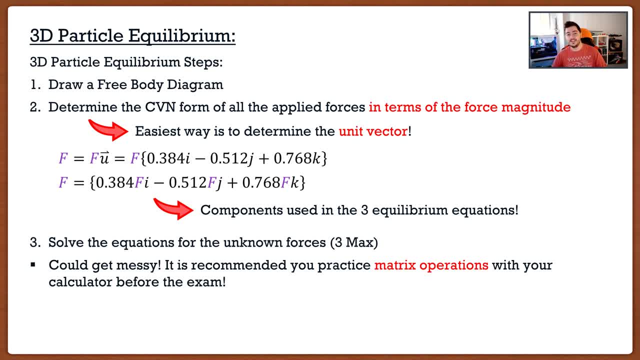 some time to yourself. i spent most of first year playing video games, if i'm being honest, and it helps. you want to find a way to manage your stress levels. if you can't- if you're too stressed, you can't really focus on things- then nothing really absorbs into you. so if you guys are finding